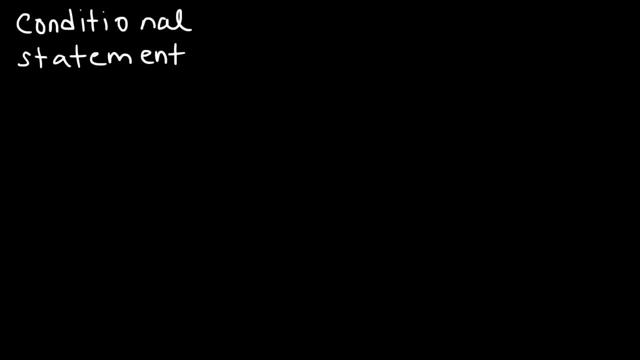 And the simplest way to describe it is as follows: If P, then Q. That is a conditional statement. So let's say, if you live in Los Angeles, then you live in California. That's an example of a conditional statement. The part that comes after the if which is denoted by P. that is the hypothesis. 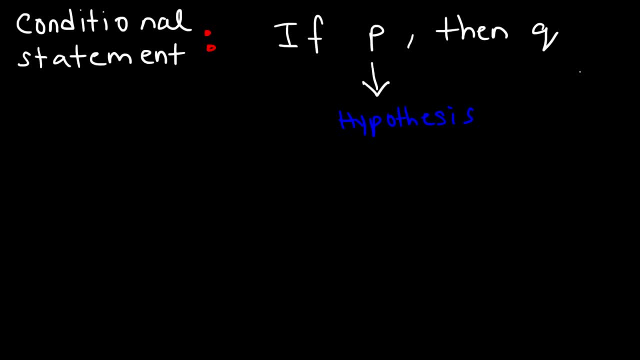 The stuff that comes after the if is the hypothesis. The stuff that comes after Q is known as the conclusion. Now you need to be familiar with the symbols. that is associated with negation. So this symbol means not P. So, for example, let's say it is sunny outside. 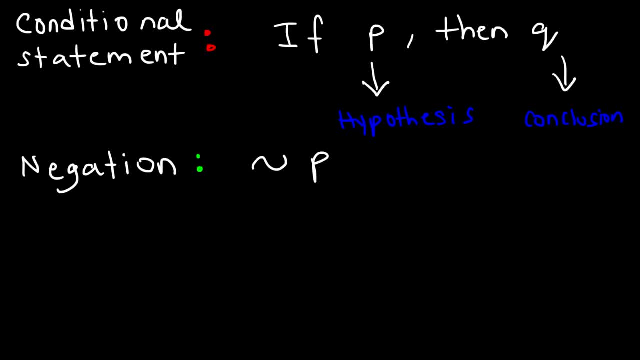 The negation of that symbol is P. So if you see this symbol, it just means it's not happening. It's a negation. Now what about the converse? What is the converse of the original conditional statement? The converse is basically the reverse of the conditional statement. 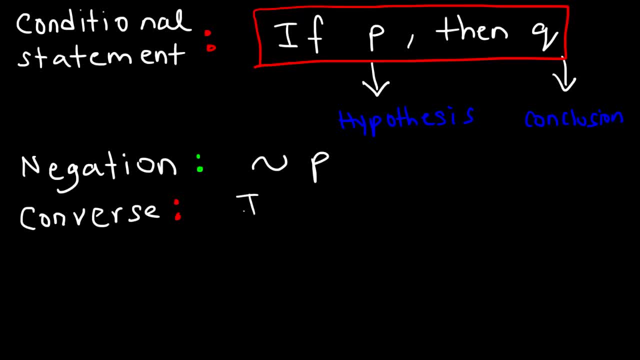 So you just got to switch Q and P. So if Q, Then P. That is the converse. If the conditional statement is true and if the converse is true, what you have is a biconditional statement. But the converse is not always true. 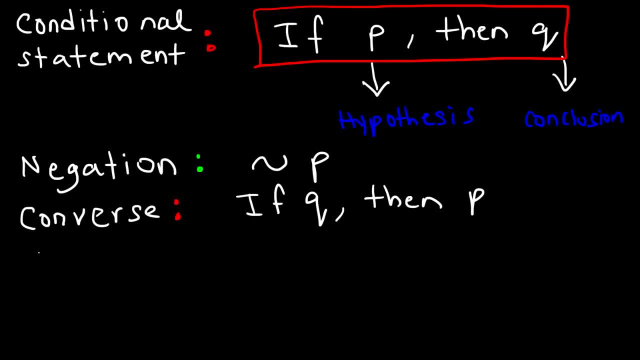 Sometimes it's true, sometimes it's not. The next term you need to be familiar with is the inverse. Now, the inverse is simply the negation of the conditional statement. If not P, then not Q. So that's the inverse. 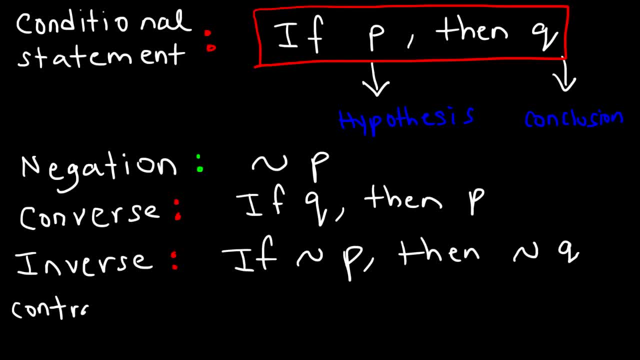 The last one you need to be familiar with is the contrapositive. The contrapositive is basically the reverse negation of the conditional statement. If not Q, then not Q. If not Q, then not Q. If not Q, then not Q. 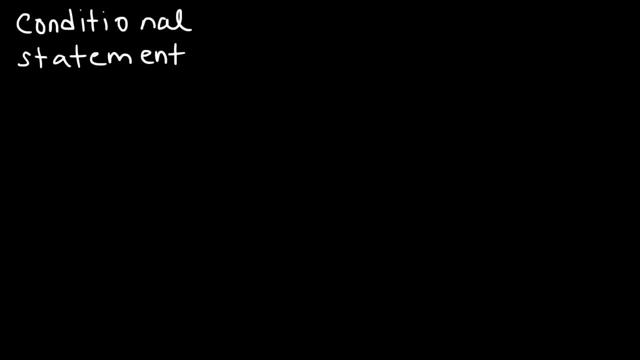 And the simplest way to describe it is as follows: If P, then Q. That is a conditional statement. So let's say, if you live in Los Angeles, then you live in California. That's an example of a conditional statement. The part that comes after the if which is denoted by P. that is the hypothesis. 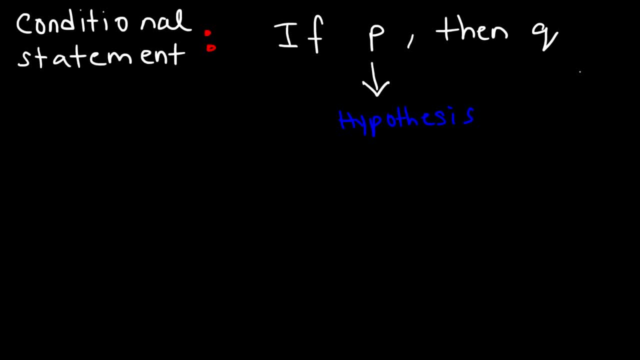 The stuff that comes after the if is the hypothesis. The stuff that comes after Q is known as the conclusion. Now you need to be familiar with the symbols. that is associated with negation. So this symbol means not P. So, for example, let's say it is sunny outside. 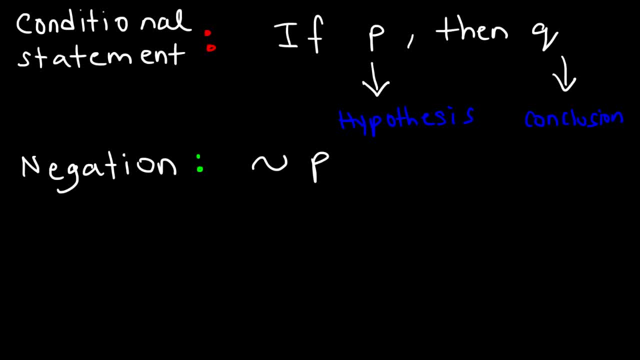 The negation of that. So if you see this symbol, it just means it's not happening. It's a negation. Now what about the converse? What is the converse of the original conditional statement? The converse is basically the reverse of the conditional statement. 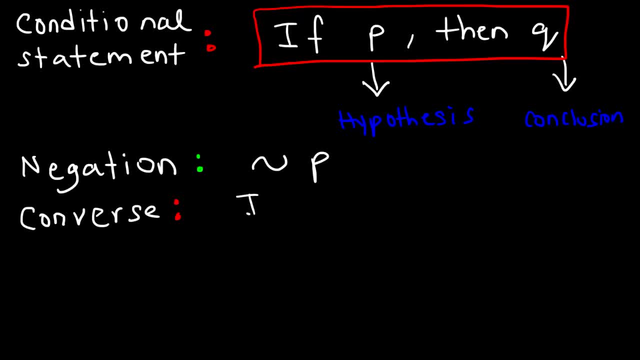 So you just got to switch Q and P. So if Q, Then P. That is the converse. If the conditional statement is true and if the converse is true, what you have is a biconditional statement. But the converse is not always true. 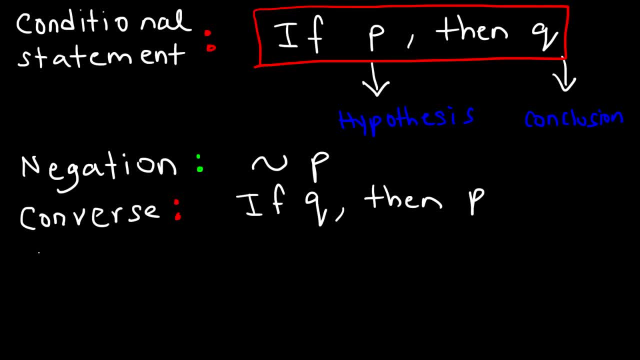 Sometimes it's true, sometimes it's not. The next term you need to be familiar with is the inverse. Now, the inverse is simply the negation of the conditional statement. If not P, then not Q. So that's the inverse. 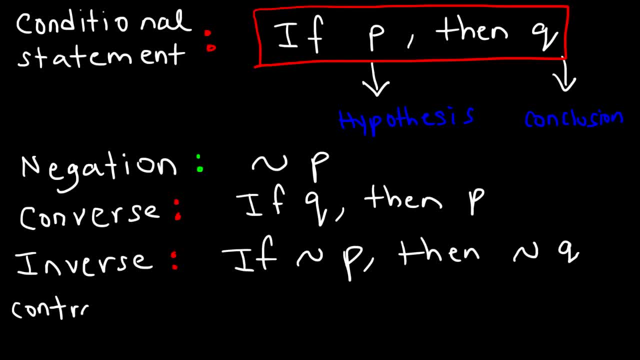 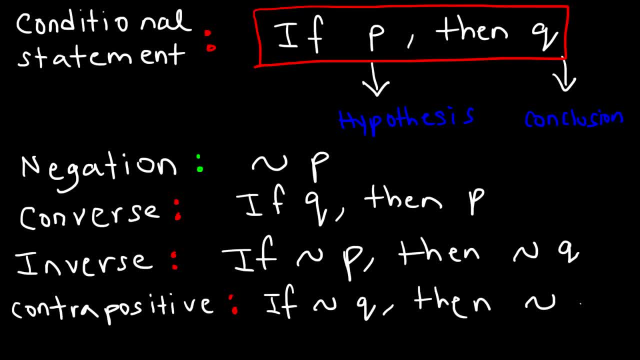 If not Q, then not Q, If not Q, then not Q, If not Q, then not P, And I'll give you some examples of that. And finally, we talked about the biconditional statement. In a biconditional statement, what you have is it occurs when the conditional statement and the converse have the same true value. 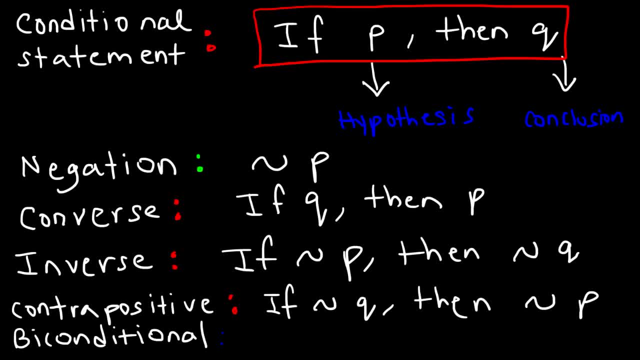 So if the conditional statement is true and if the converse is true, then you have a biconditional statement In the conditional statement, if P then Q. In a biconditional statement it can go both ways. So if P then Q, or if Q then P. 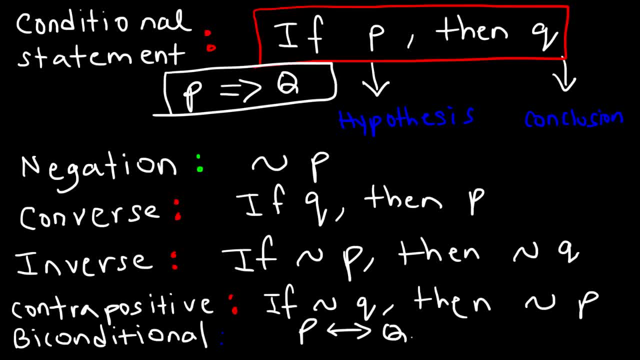 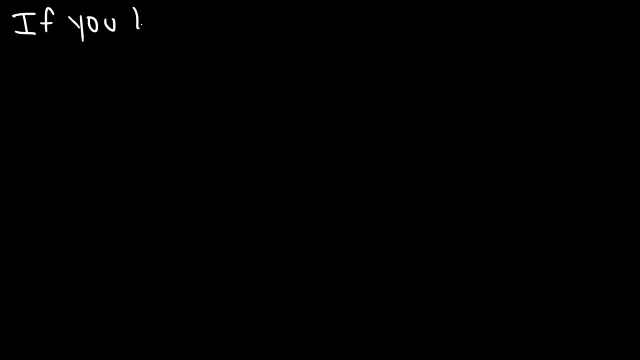 Both will be true or both will be false. That's a biconditional statement. So let's try an example. Let's try an example: If you live in Los Angeles, then you live in California. So this is the conditional statement. 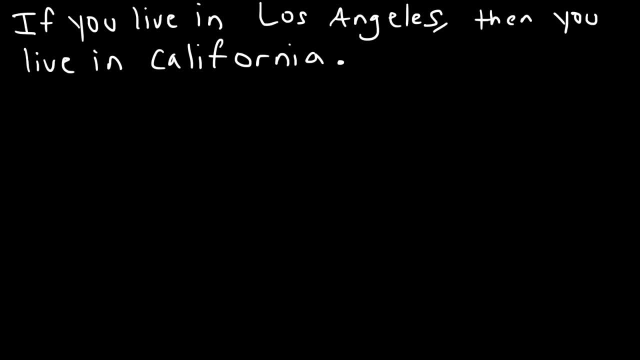 Now, what is the hypothesis and what is the conclusion? The hypothesis is the stuff that comes after the if part, So the hypothesis is living in Los Angeles, The conclusion is living in California. Now how can we write this? 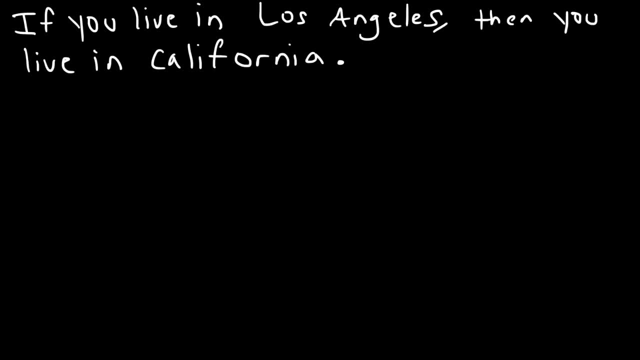 How can we write the converse and the inverse, in addition to the contrapositive of this statement? So right now, keep in mind: the hypothesis is P, So P is living in Los Angeles and Q is living in California. So right now we have: if P, then Q. 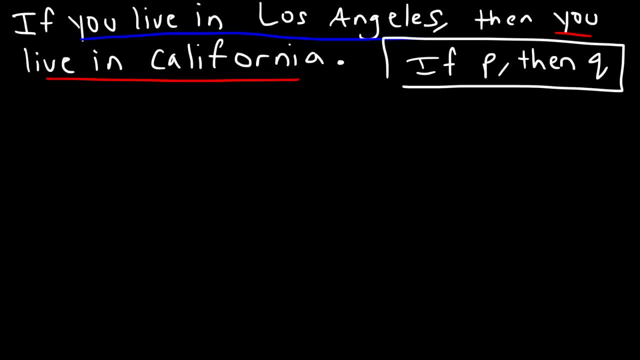 So that's the conditional statement. To write the converse, we need to recall that the converse is the reverse of the conditional statement. If Q, then P. So what we need to do is switch the second part of the sentence with the first part. 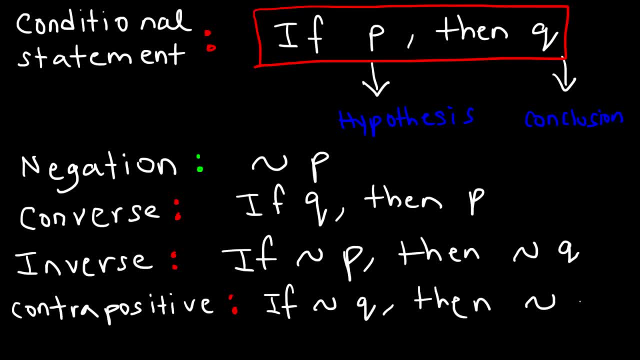 If not Q, then not Q, If not Q, then not Q, If not Q, then not P, And I'll give you some examples of that. And finally, we talked about the biconditional statement. In a biconditional statement, what you have is it occurs when the conditional statement and the converse have the same true value. 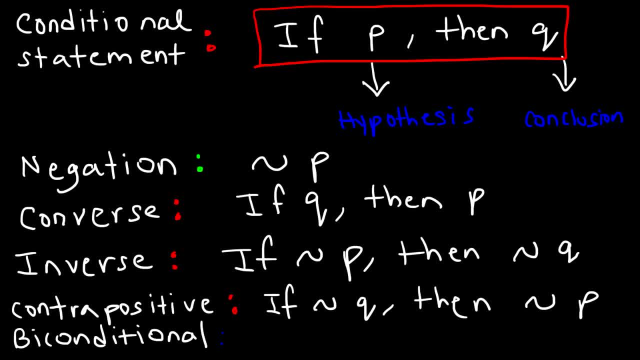 So if the conditional statement is true and if the converse is true, then you have a biconditional statement In the conditional statement. if P, then Q. If the conditional statement is true and if the converse is true, then you have a biconditional statement. 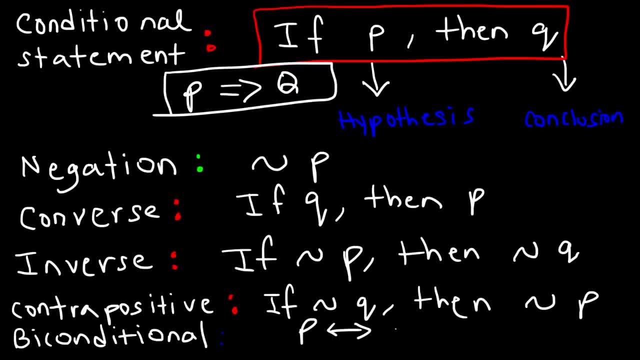 In a biconditional statement it can go both ways. So if P then Q, or if Q then P, Both will be true or both will be false. That's a biconditional statement. So let's try an example. 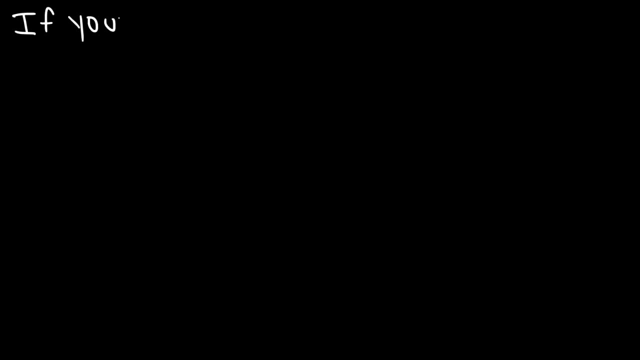 Let's try an example: If you live in Los Angeles, then you live in California. So this is the conditional statement. Now, what is the hypothesis and what is the conclusion? The hypothesis is the stuff that comes after the if part. 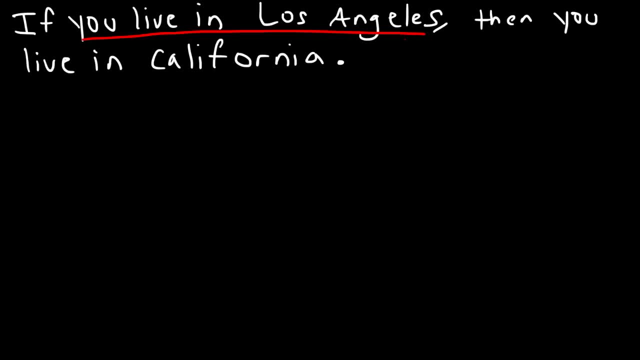 So the hypothesis is living in Los Angeles, The conclusion is living in California. Now, how can we write this? How can we write the converse and the inverse, in addition to the contrapositive of this statement? So right now, keep in mind: the hypothesis is P. 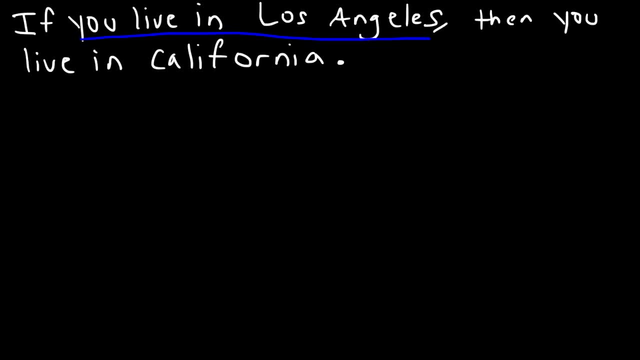 So P is living in Los Angeles and Q is living in California. So right now we have: if P, then Q, So that's the conditional statement To write the converse. we need to recall that the converse is the reverse of the conditional statement. 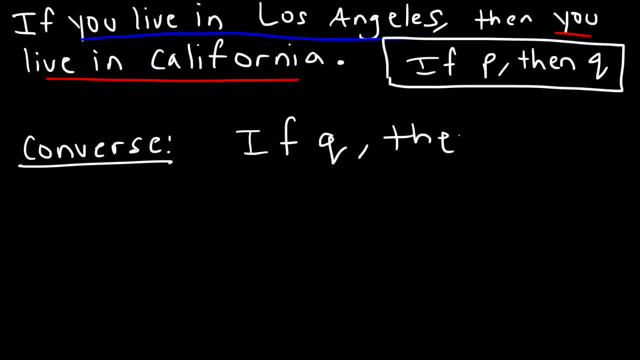 If Q, then P. So what we need to do is switch the second part of the sentence with the first part. So, therefore, the converse will be as follows: If you live in California, California, California, California, then you live in Los Angeles. 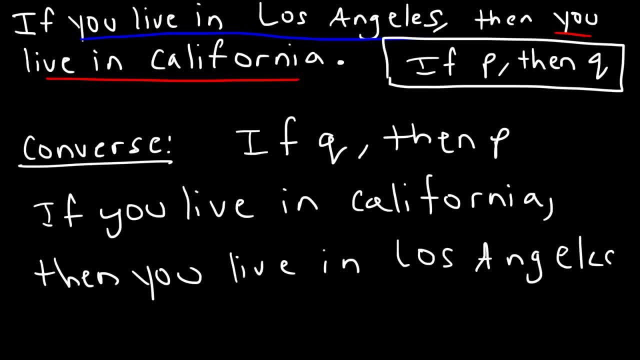 So that is the converse. Now, is the converse a true statement or is it a false statement? Right now, we're assuming that the conditional statement is true, But the converse is a false statement. Someone who lives in California doesn't have to live in Los Angeles. 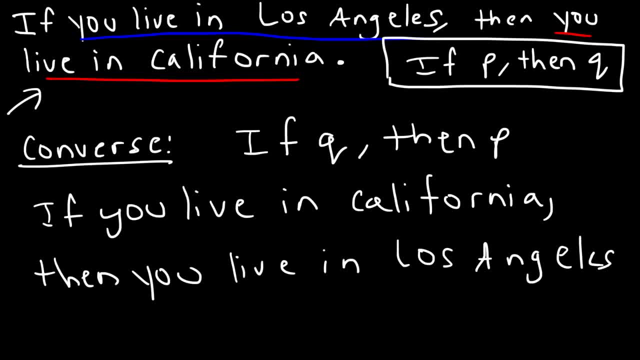 They can live in Los Angeles, They can live in Sacramento, They can live in San Francisco or San Diego, So the converse is false. So if you have a true conditional statement and a false converse statement, then this is not a biconditional statement. 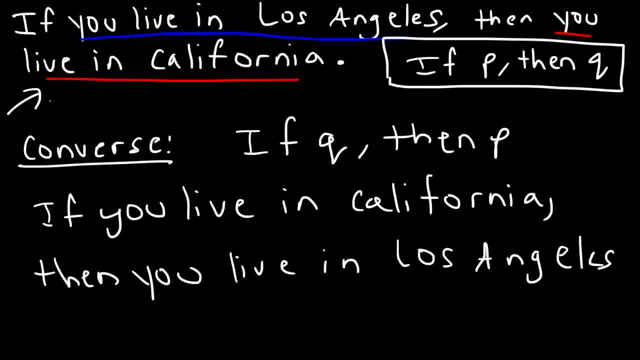 If the converse was true and if the conditional statement assuming that's true as well, then we would have a biconditional statement. Now let's write the inverse. So the converse is the negation of the conditional statement. So recall that the inverse is simply the negation of the condition of the conditional statement. 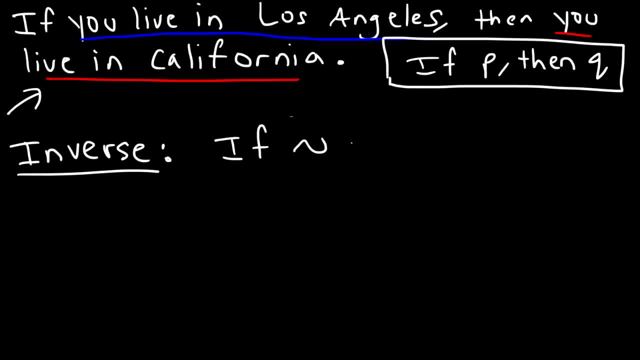 Excuse me. So if not P, then not Q. So the sentence will be as follows: If you don't live in Los Angeles, I'm going to write L? A for Los Angeles. Then you don't live in California. 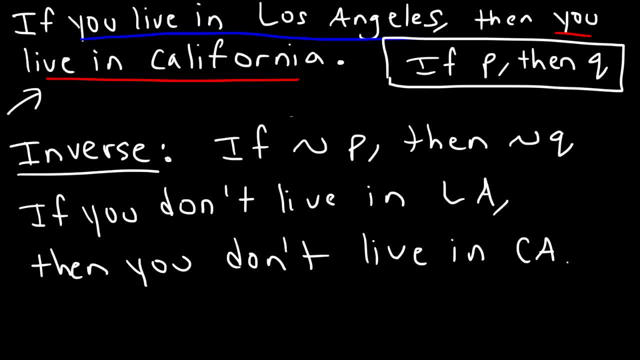 So I'm going to write C A for California. So that's the inverse: If you don't live in Los Angeles, you don't live in California. So you don't reverse the sentence, You simply negate the sentence from being yes to no. 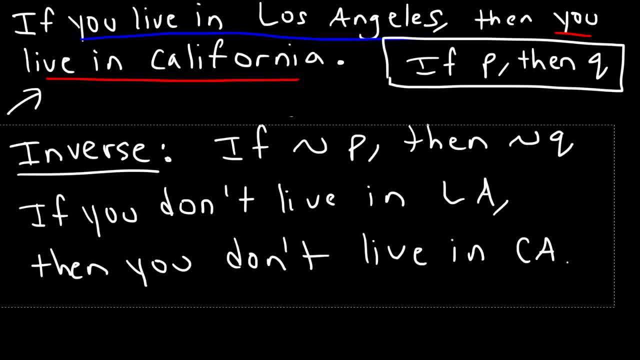 Now, what about the contrapositive? Oh, by the way, is the inverse true? If you don't live in LA, then you don't live in California. what would you say? Well, just because you don't live in LA doesn't mean you don't live in California. 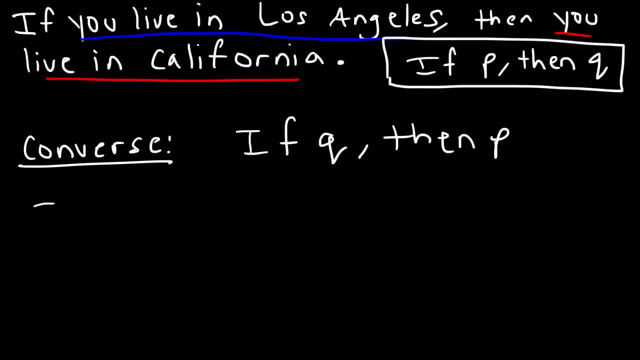 So, therefore, the converse will be as follows: If you live in California, California, then you live in Los Angeles. So that is the converse. Now, is the converse a true statement or is it a false statement? Right now, we're assuming that the conditional statement is true. 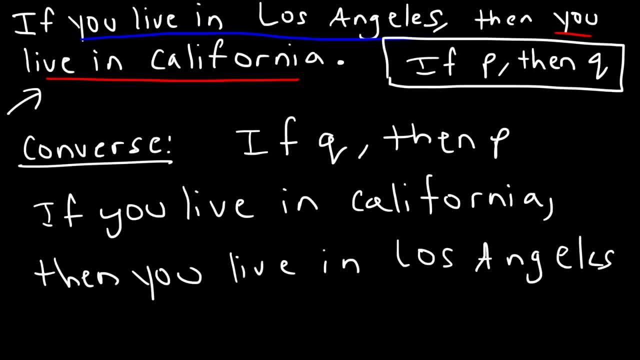 But the converse is a false statement. Someone who lives in California doesn't have to live in Los Angeles. They could live in Sacramento, They could live in San Francisco or San Diego. So the converse is false. So if you have a true conditional statement and a false converse statement, 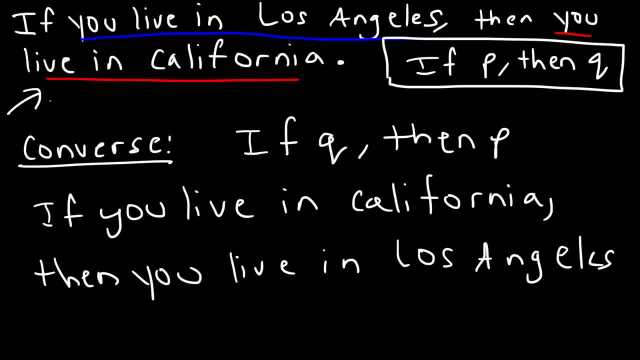 then this is not a biconditional statement. If the converse was true and if the conditional statement, assuming that's true as well- then we would have a biconditional statement. Now let's write the converse. So if not P, then not Q. 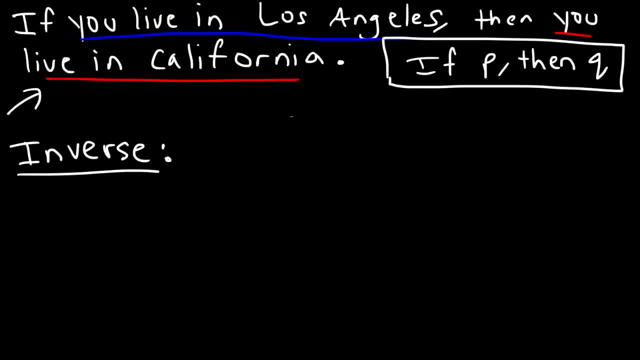 So recall that the inverse is simply the negation of the conditional statement. So if not P, then not Q. So the sentence will be as follows: If you don't live in Los Angeles, I'm going to write LA for Los Angeles. 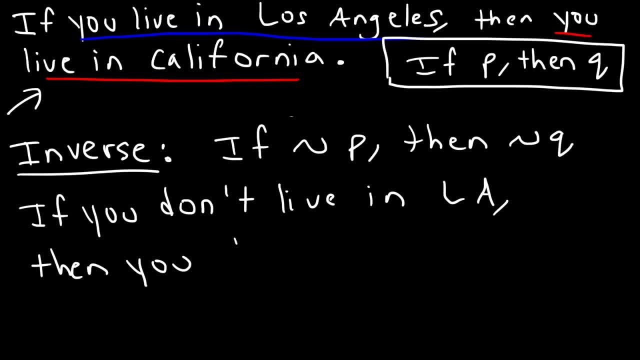 then you don't live in California. So I'm going to write CA for California. So that's the inverse: If you don't live in Los Angeles, you don't live in California. So you don't reverse the sentence, You simply negate the sentence from being yes to no. 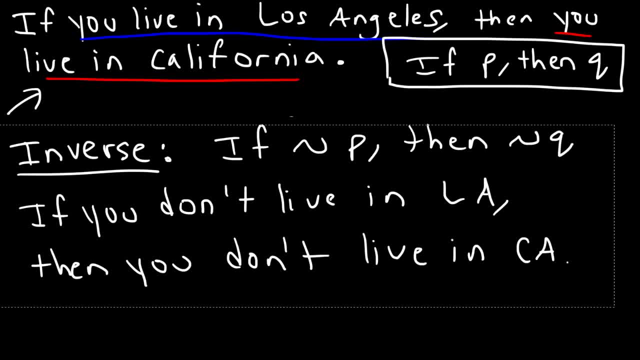 Now, what about the contrapositive? Oh, by the way, is the inverse true or false? If you don't live in LA, then you don't live in California. What would you say? Well, just because you don't live in LA doesn't mean you don't live in California. 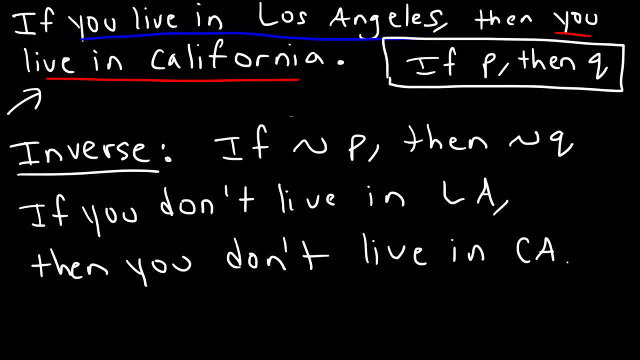 Because you can live in San Francisco, which is not in LA but still within the state of California. So in this case the inverse is false. It turns out that if the converse is false, the inverse is going to be false. Those two have the same true value. 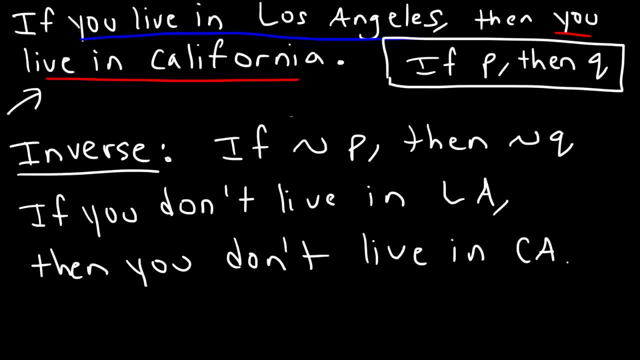 If the converse is true, then the inverse is false. So if you don't live in LA, then you don't live in California. The inverse is going to be true as well. Now let's write the contrapositive statement. So remember: the contrapositive is basically the reverse negation of the conditional statement. 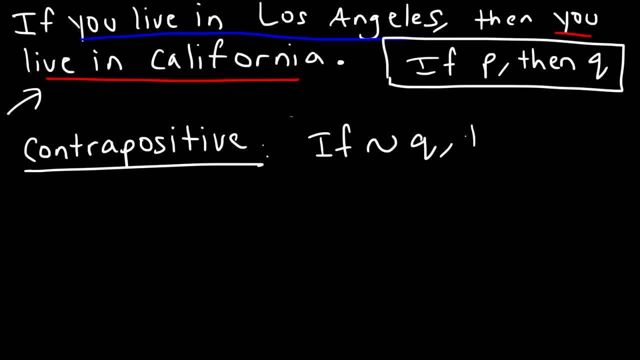 And it says: if not Q, then not P. So we've got to reverse it and negate it. So the sentence will be as follows: If you don't live in California, then you don't live in Los Angeles. Now, is that a true statement. 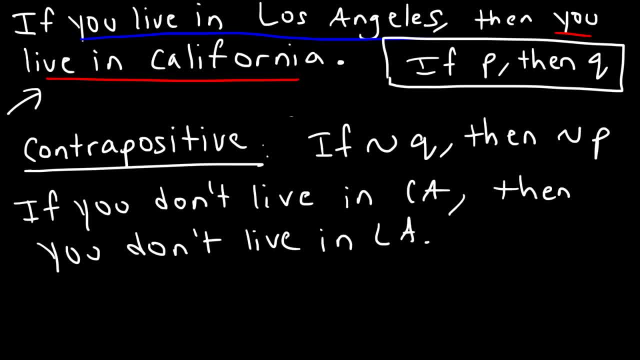 It turns out that it is Because if you don't live in the state of California, you can't live inside a city within California, which is LA. Now it turns out that if the conditional statement is true, then the contrapositive will be true. 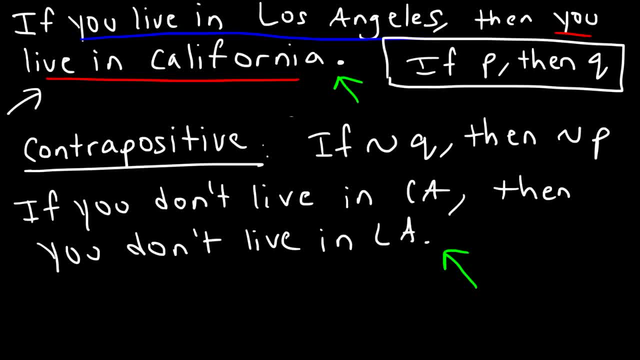 And if the conditional statement is false, the contrapositive will be false. So the conditional statement and the contrapositive will always have the same true value. They will always be the same, In the same way as the converse and the inverse are always the same. 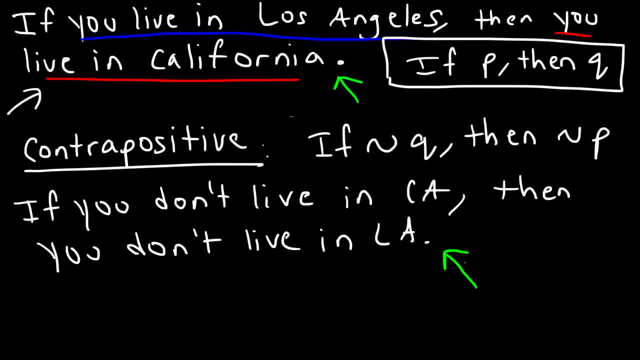 Any time you have a reverse negation of something, it's like a double reverse. It's going to take you back to the original value. And that's what's happening with the contrapositive: Not only do you reverse the statements, but you negate it as well, which makes it true again. 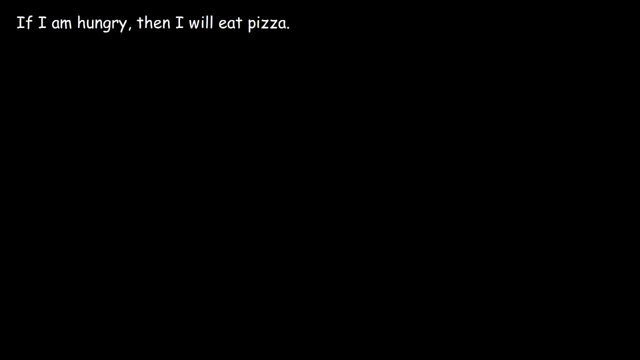 Go ahead and work on this example problem. If I am hungry, then I will eat pizza. So, given that conditional statement, write the converse, the inverse and the contrapositive. So let's start with the converse. The converse is simply the reverse of the conditional statement. 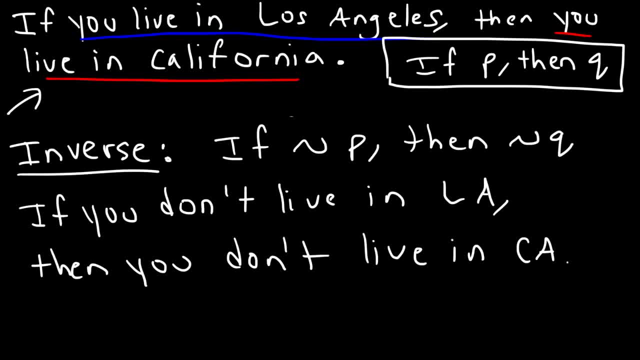 because you can live in San Francisco, which is not in LA but still within the state of California. So in this case the inverse is false. It turns out that if the converse is false, the inverse is going to be false. Those two have the same true value. 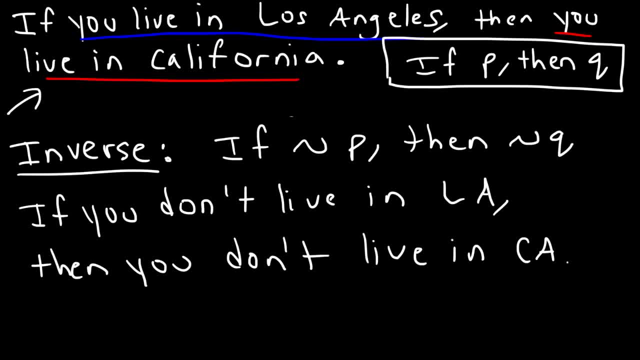 If the converse is true, then the inverse is going to be true as well. Now let's write the contrapositive statement. So remember: the contrapositive is basically the reverse negation of the conditional statement, And it says: if not, Q. 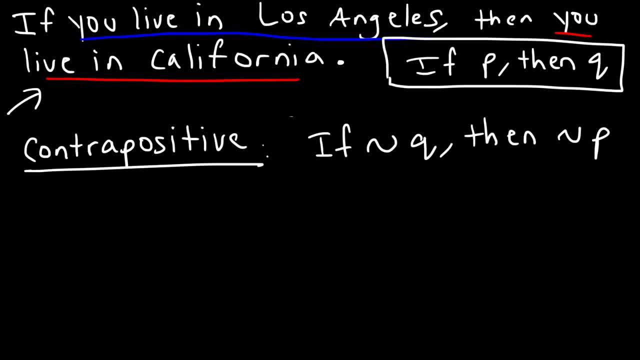 then not, not P. So we've got to reverse it and negate it. So the sentence will be as follows: If you don't live in California, then you don't live in Los Angeles. Now, is that a true statement? It turns out that it is. 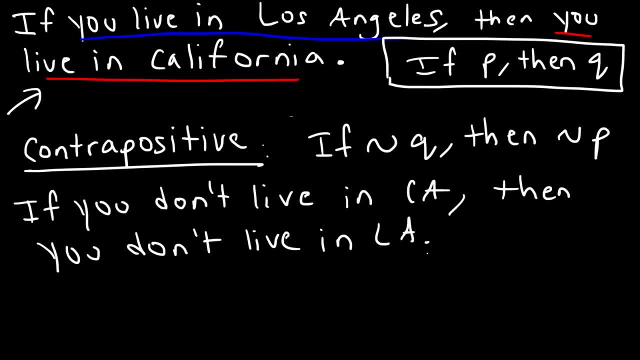 because if you don't live in the state of California, you can't live inside a city within California, which is LA. Now it turns out that if the conditional statement is true, then the contrapositive will be true, And if the conditional statement is false, 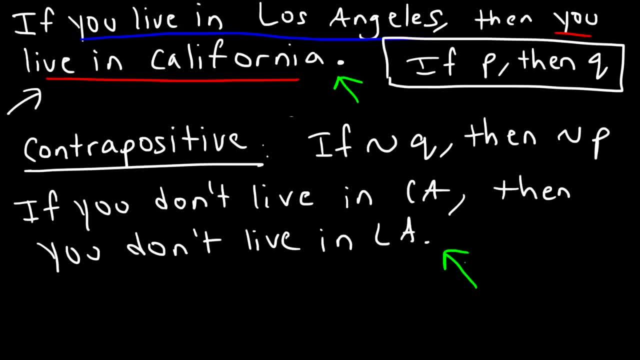 the contrapositive will be false. So the conditional statement and the contrapositive will always have the same true value. They will always be the same, In the same way as the converse and the inverse are always the same Anytime you have a reverse negation of something. 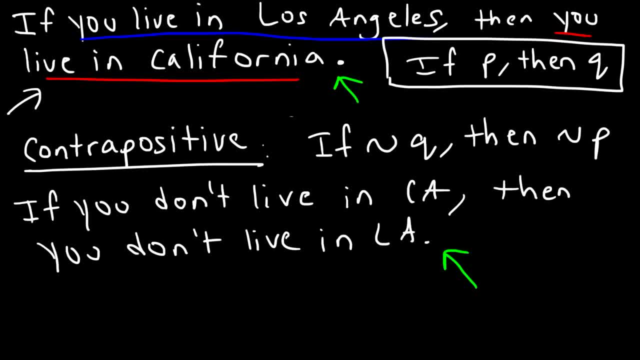 it's like a double reverse. It's going to take you back to the original value, And that's what's happening with the contrapositive: Not only do you reverse the statements, but you negate it as well, which makes it true again. 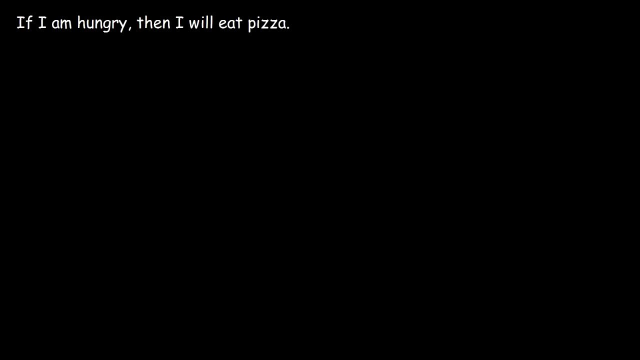 Go ahead and work on this example problem. If I am hungry, then I will eat pizza. So, given that conditional statement, write the converse, the inverse and the contrapositive. So let's start with the converse. The converse is simply the reverse.